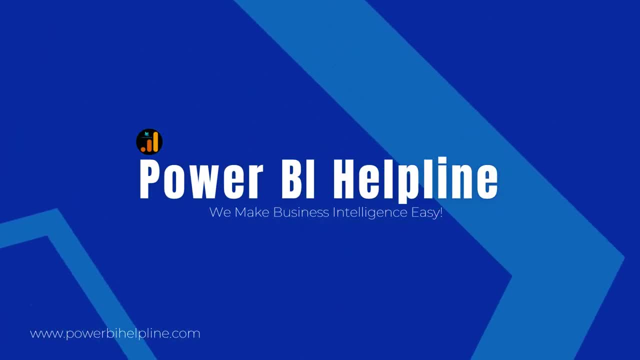 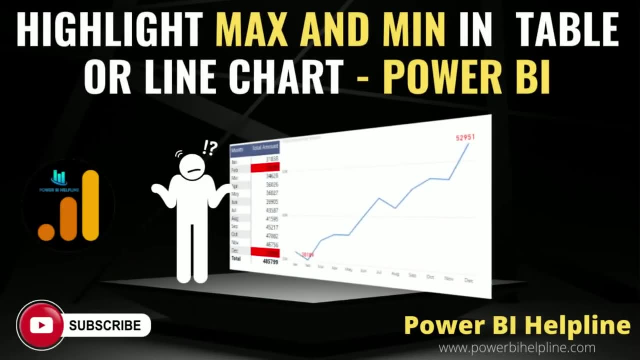 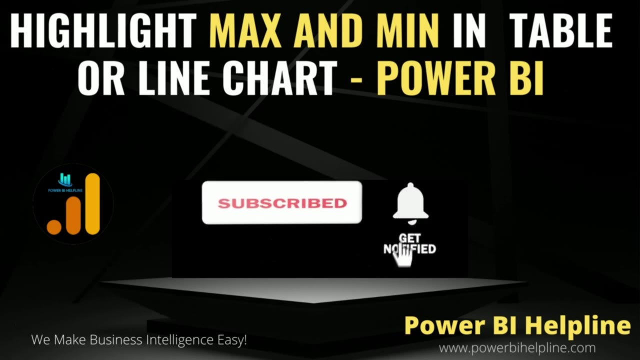 Welcome back to Power BI Helpline YouTube channel. Today in this video, we are going to explain how you can highlight maximum and minimum values in Power BI visuals. If you are visiting here for the first time, then please subscribe to this channel and hit the bell icon to get notified. 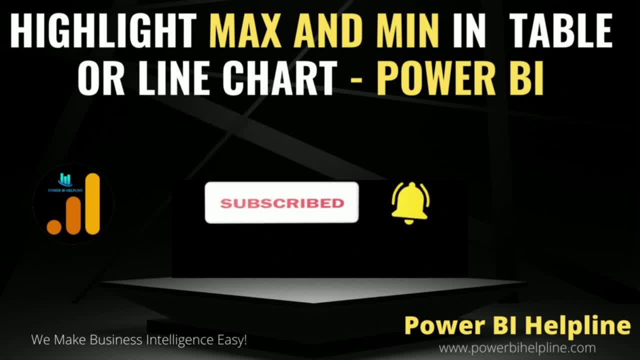 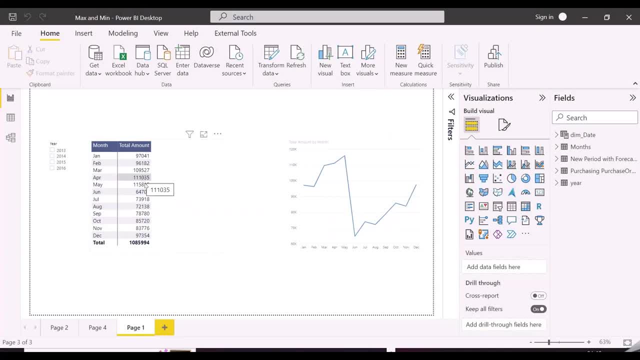 for all such interesting solutions in Power BI. With that, let's check it out. For this example, we have created two visuals: a line chart and a matrix which is showing month-wise total amount. First of all, we will create two measures showing the ranks based on total amount. 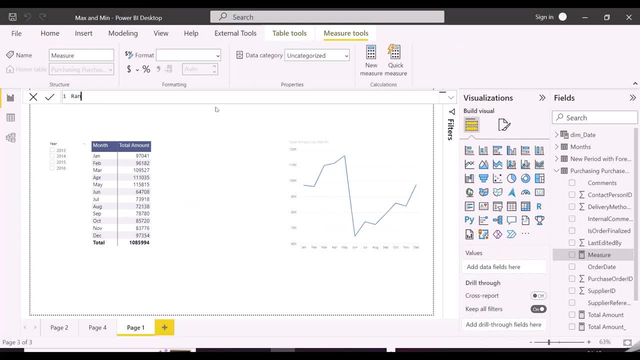 One measure will be created based on ascending order and another is on descending order, And then, finally, we will use these two measures to solve this particular problem. Since our month name is sorted by month number, we also need to include month number inside all selected argument. This measure will assign rank 1 to 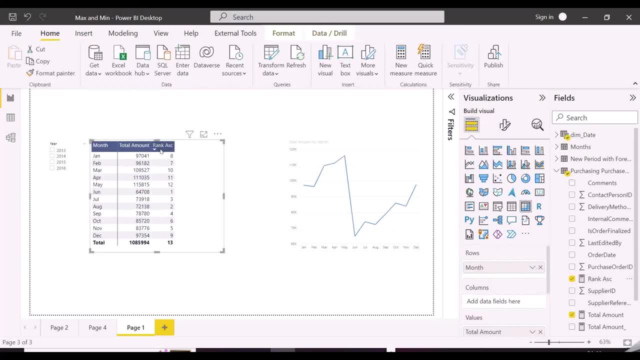 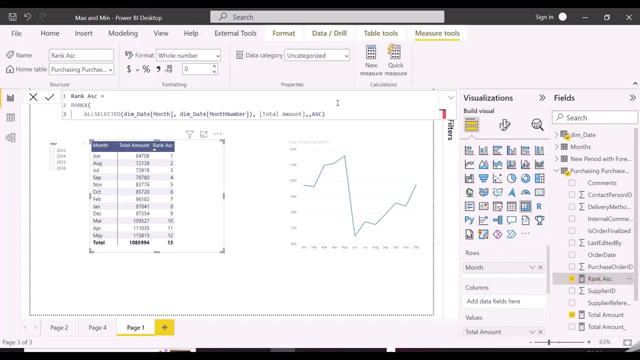 the number of ranks that are listed in Power BI. The lowest sales amount, month. As that you can see, it is showing rank 1 for the lowest total amount in our matrix visual. Now we will create another measure with descending order and finally, 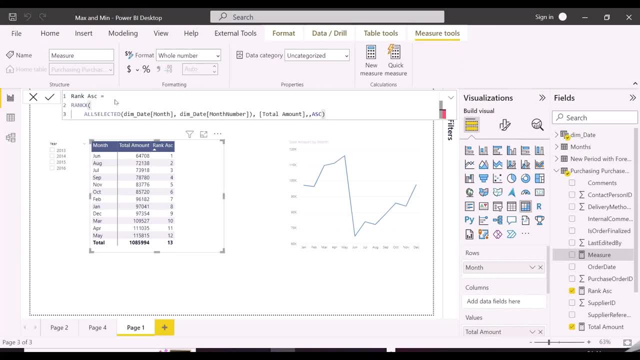 we'll show you the trick as how you can use these two measures to highlight maximum and minimum in Power BI visuals. As said, we have copied the same measure and changing the order from ascending to descending. We don't need to keep these two measures inside your visual, but I am keeping 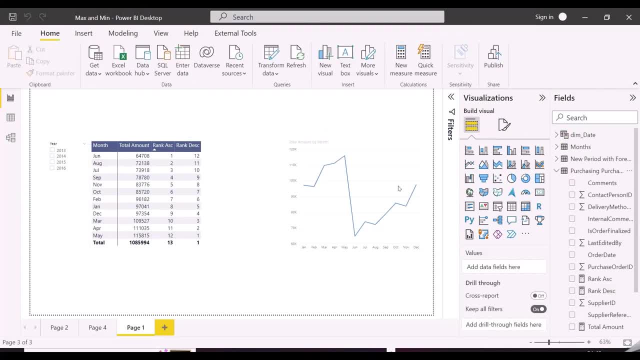 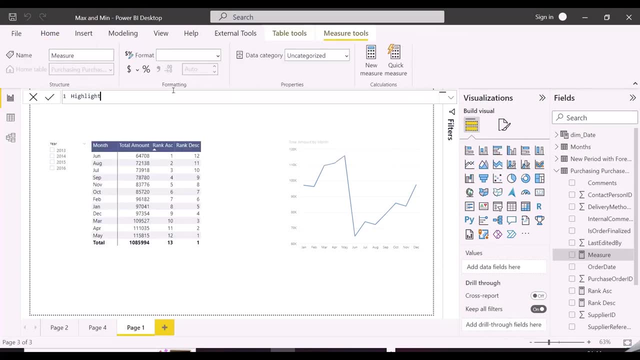 them here so that it will be easy to understand The next measure for highlight max and min Now, since we know that one measure is showing rank 1 for the lowest amount, while the other is showing rank 1 for the highest amount. 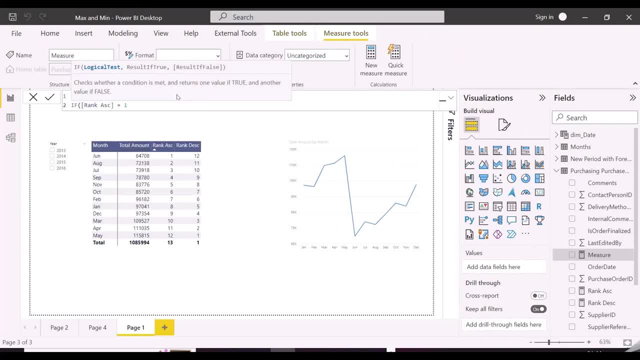 So here I am creating a measure which will validate if there is rank 1 from any of the measures output, then show red color or show a transparent color. The hex code for the transparent color is 6F and 00.. And now we are done with our workaround and we'll apply this. 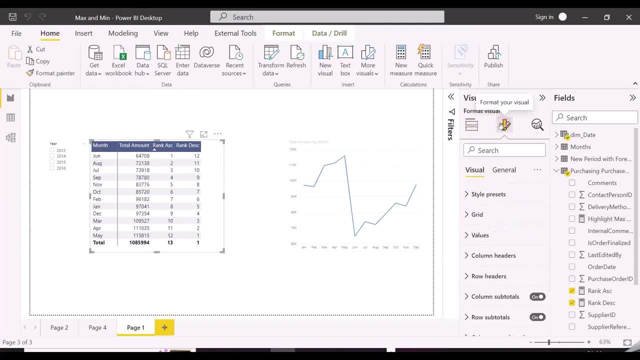 to this matrix and line chart visual. In this example we will use the same measure to show max and min. For this example, I am formatting the background color of max and min, but you can also do this with font color From format style of the background formatting you need to select.